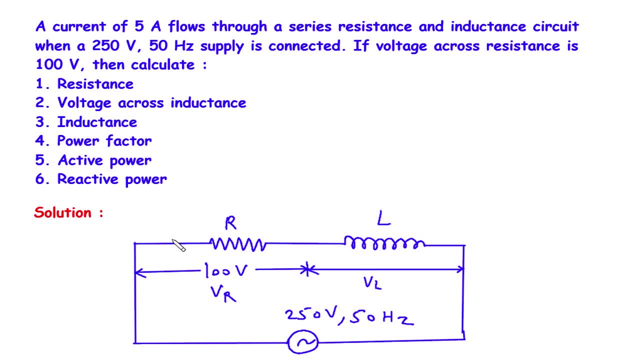 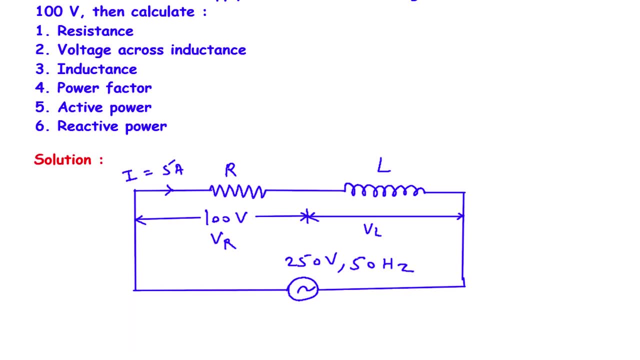 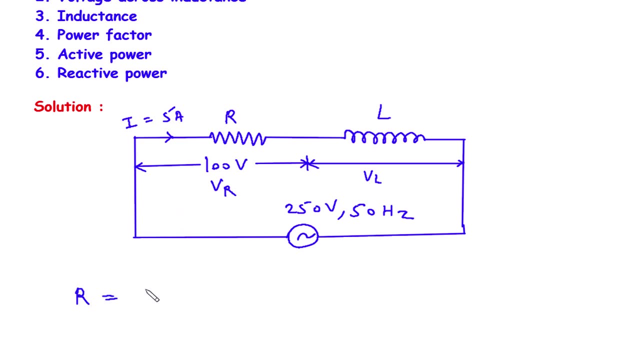 we have to find the value of current. Here we can see the value of current is also. given This current I is equal to 5A. Now we have the value of current and voltage. By using Ohm's law we can find the value of resistance. So resistance R is equal to VR divided by I. 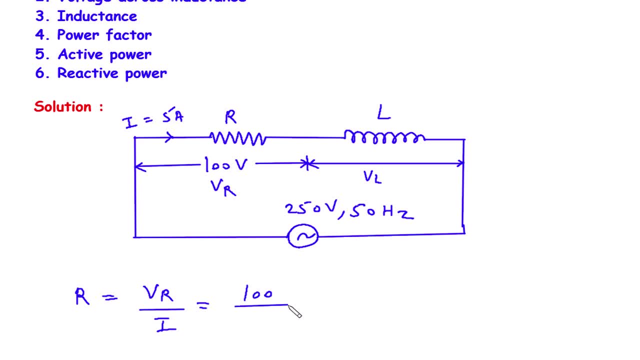 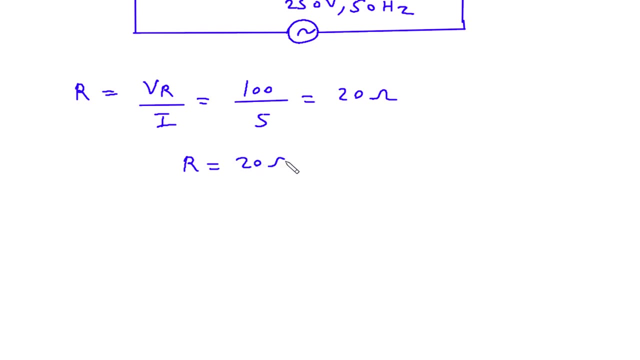 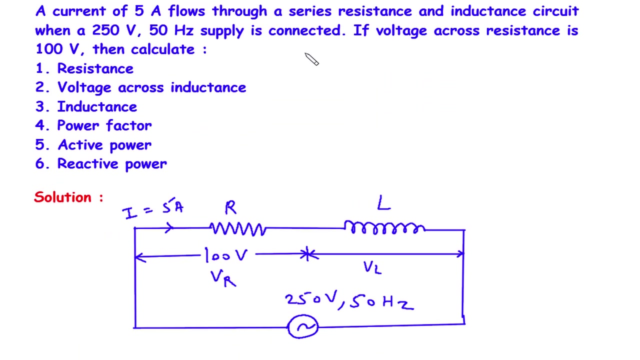 The value of VR is 100 and the value of current I is 5.. this will be 20- 20 ohms. This is the value of resistance. R R is equal to 20 ohm. Then next next is we have to find the voltage across inductance. So, to find voltage across inductance, 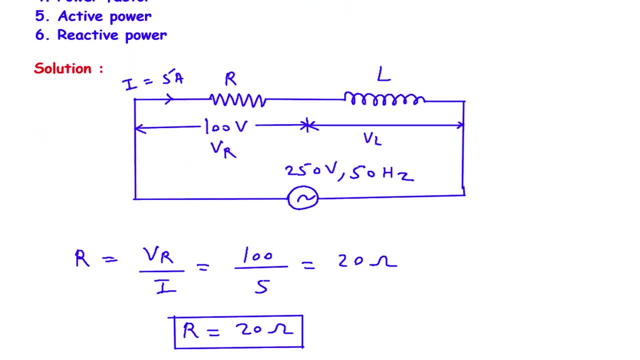 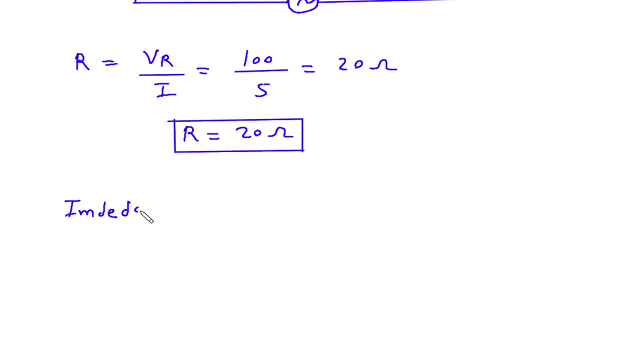 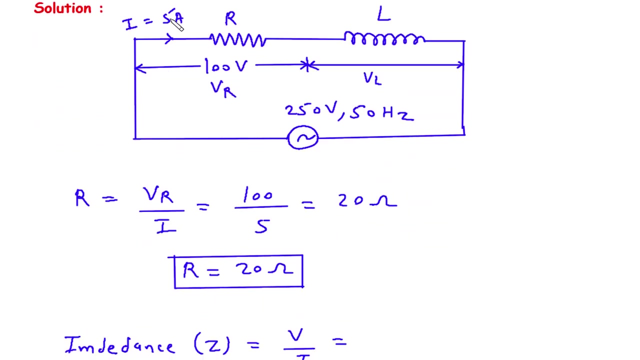 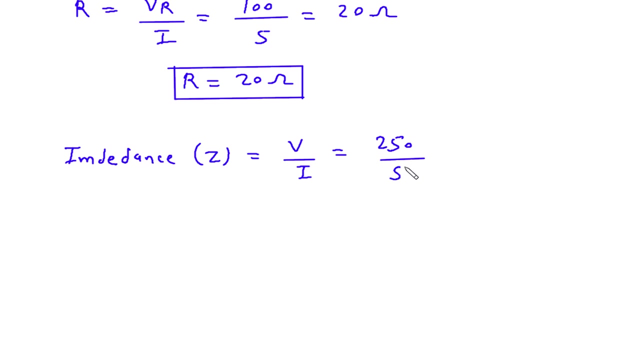 first of all we have to find impedance. Now, impedance Z is equal to V by I. The value of voltage is given, it is 250 volts and the value of current is 5 ampere. So 250 divided by 5. So this will be 5050 and its unit will be ohm. So therefore, impedance Z is equal. 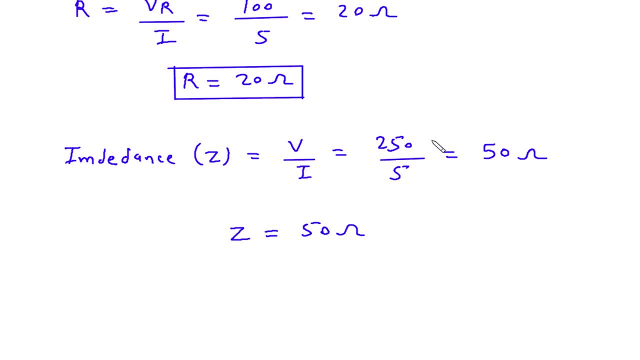 to 50 ohm. Now, by using the value of Z and R, we can find the value of XL, because Z is equal to under root of R square plus XL square. Now if we take square on both side, then this will be: Z square is equal to R square plus XL. 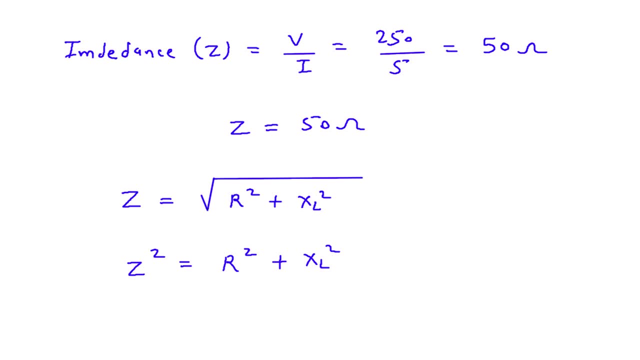 square. This under root will be cancelled with this square. this square, We are taking square on both side, So this will be Z square and here on right side, this under root will get cancelled. Now we have the value of Z and R, So we have to find the value of XL, So from here we can say XL. 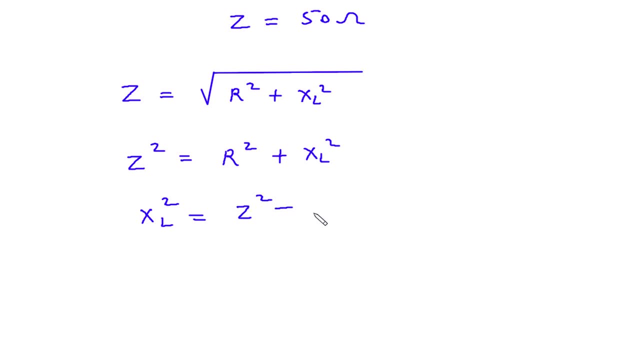 square is equal to Z square minus R square. or we can say: XL is equal to under root of Z square minus R square. Now we will substitute the value of Z and R The value of Z, 50 ohm. so this will be 50 minus. this will be 50 square. 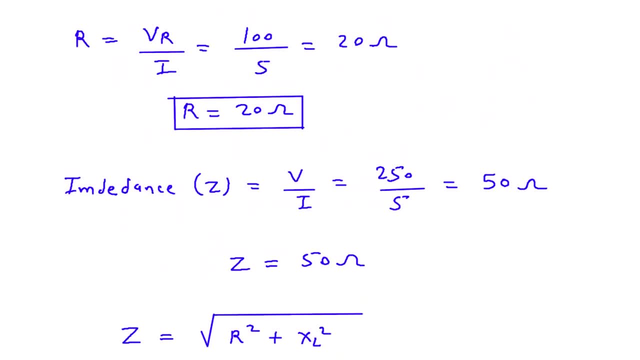 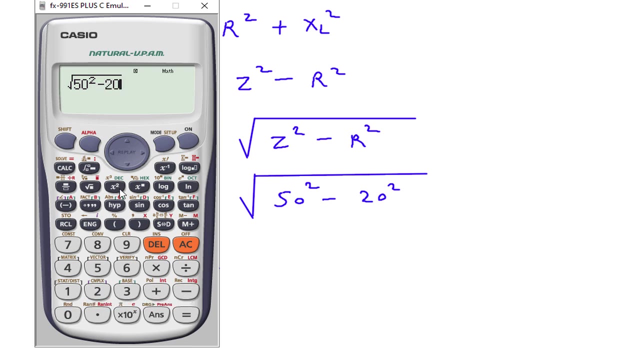 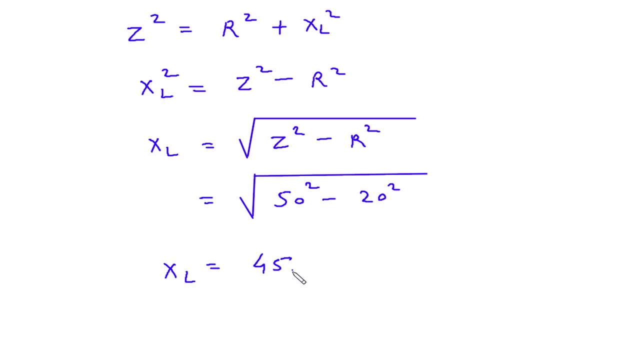 So this will be 50 ohm, so this will be 50 minus this will be 50 square. then minus R square will be 20 square, So this will be 20 square. So therefore, xl is equal to under root of 50 square minus 20 square, So it is 45.82, 45.82 ohms. This. 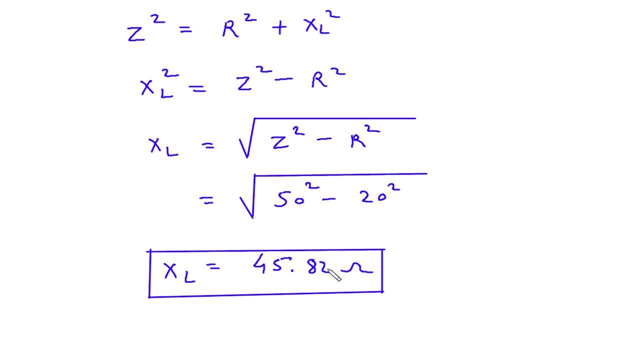 is the value of inductive reactance. The unit of inductive reactance is ohm. Then next is from here we can find the value of inductance, because inductance, inductive reactance, is equal to 2 pi f into L. So from here, L is equal to xl divided by 2 pi f. Here the value. 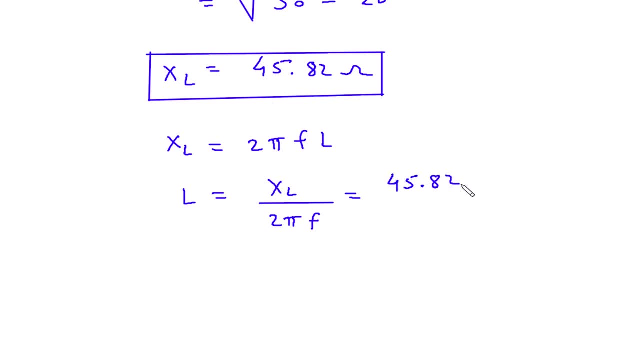 of xl is 45.82 divided by 2 pi f. So this is the value of inductive reactance. So this is the value of inductive reactance. So this is the value of inductive reactance. So this: 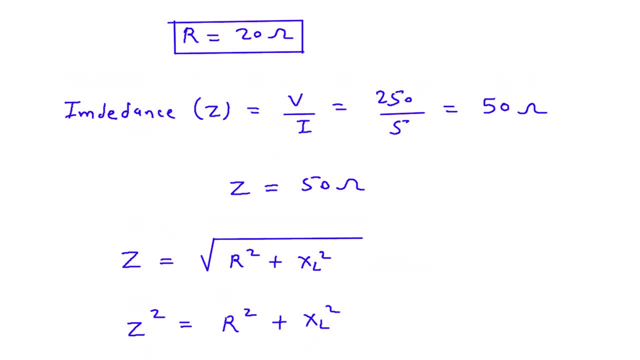 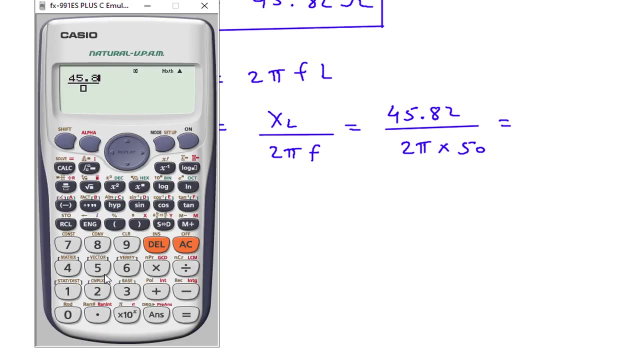 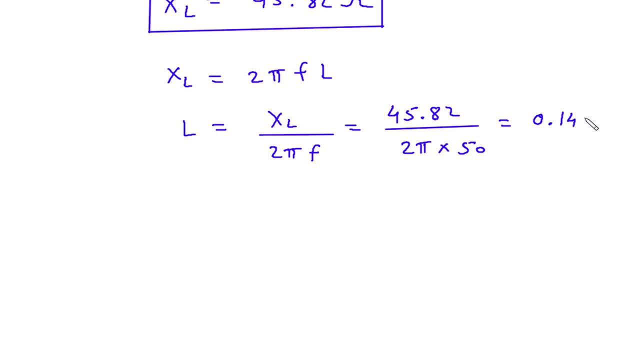 two pi multiplied by f. f is the frequency and its value is where we can see. frequency is 50 hertz, So this will be 50.. Now, if we calculate this, so this will be 45.82 divided by 2, multiplied by pi multiplied by 15.. So it is 0.145, 0.145.. This is the inductance. 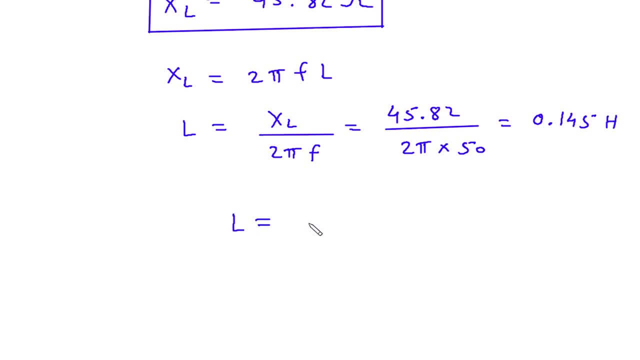 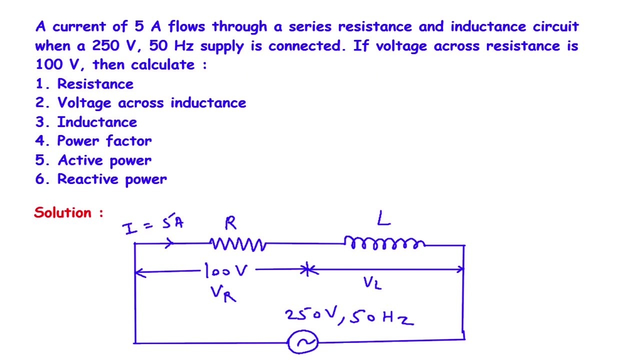 so its unit will be Henry. So therefore L is equal to 0.145 Henry. Now resistance value, then voltage across inductance. Next we have to find- we already find- the value of resistance and inductance. Next we have to find voltage across inductance. 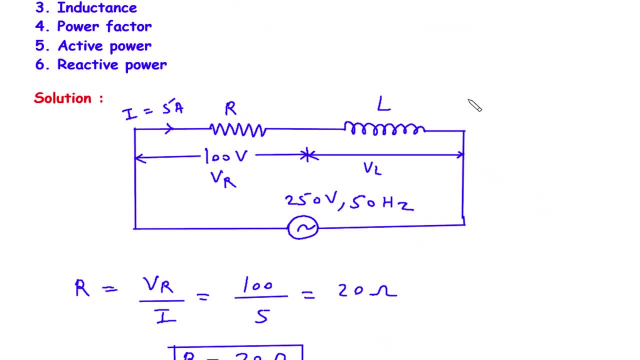 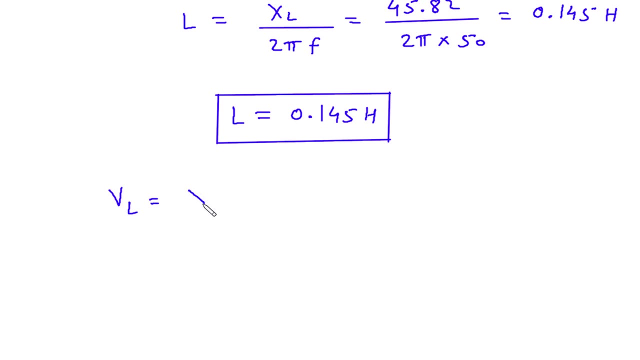 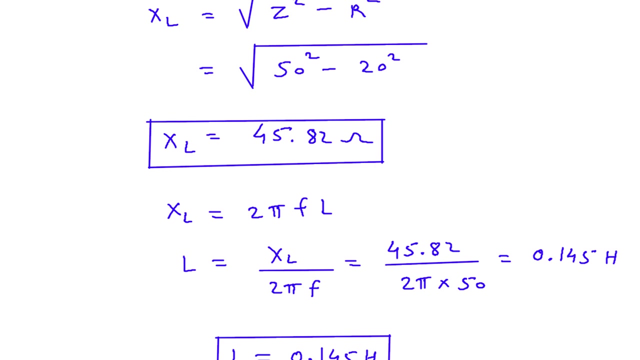 So voltage across inductance will be: VL is equal to. VL is equal to XL into I, So VL is equal to XL, XL into I. the value of inductive reactance is 45.82,, 45.82 multiplied by current. 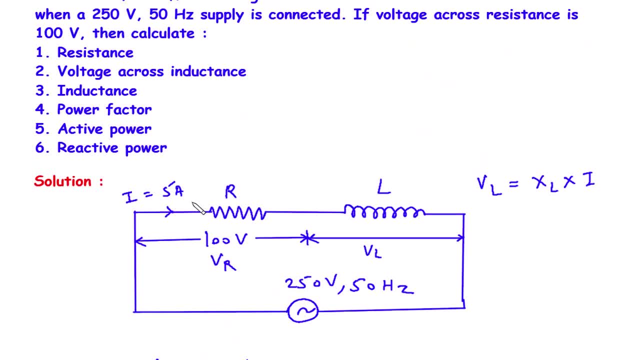 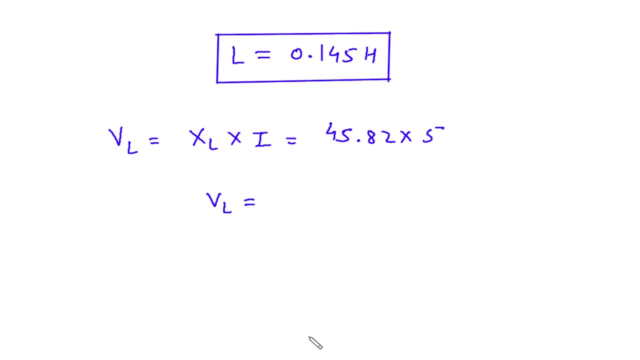 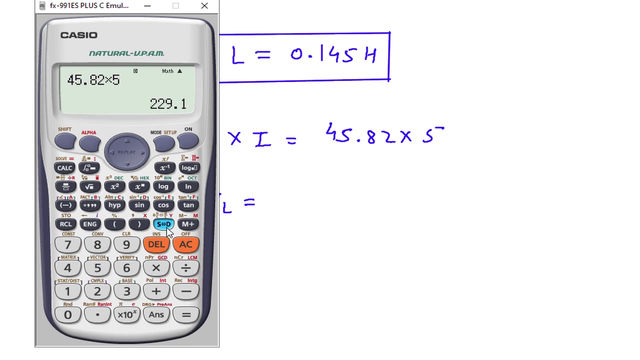 is current will be same in both resistance and inductance, because they are connected in series. So here the current is 5 ampere, So here also the current will be 5 ampere, So this will be 5.. Now if we calculate this, VL is equal to 45.82 multiplied by 5.. So it 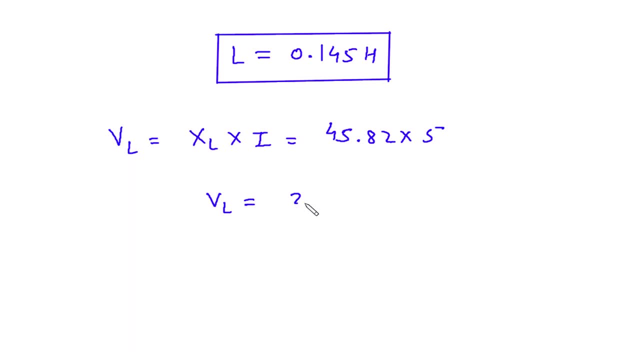 is 229.1, 229.1.. Now, this is the voltage, so its unit will be volts. OK, Now next we have to find power factor. We know that power factor is equal to. power factor is equal to cos phi and it is equal to R. 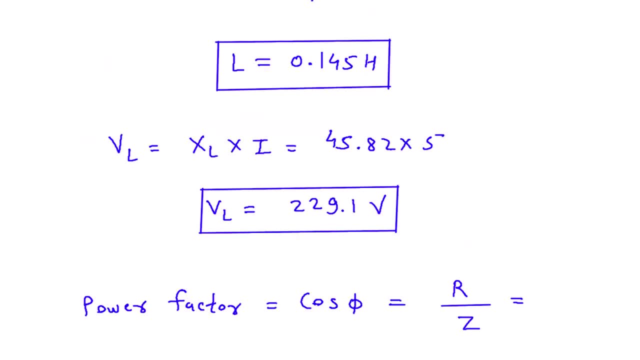 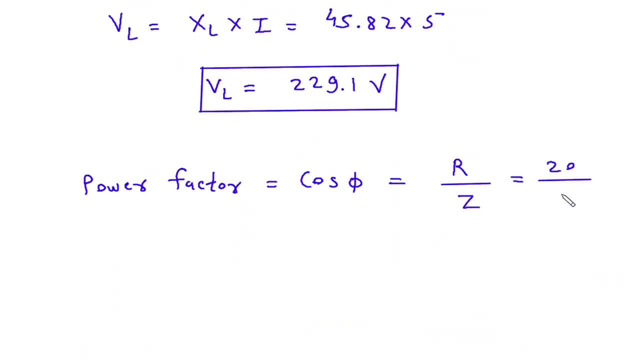 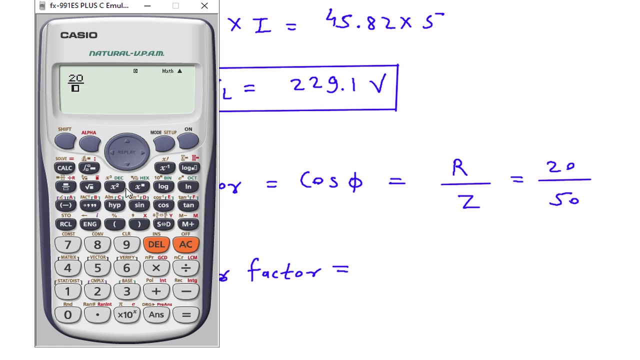 upon z. The value of resistance R is 20 ohm and the value of impedance z is 10 ohm. So audiences are energy Trent'm. There we can see. Z is equal to 50 ohm, 50 ohm. So therefore, power factor is equal to. power factor is equal to R by Z, that is 20 divided. 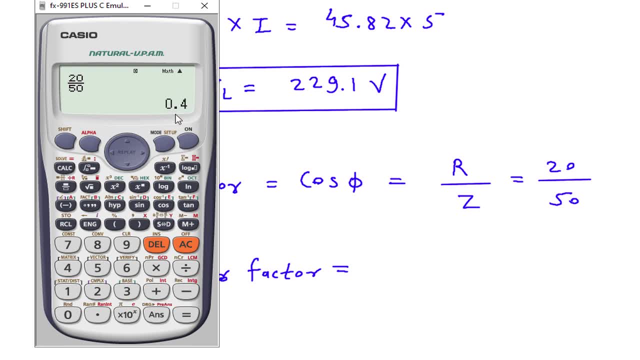 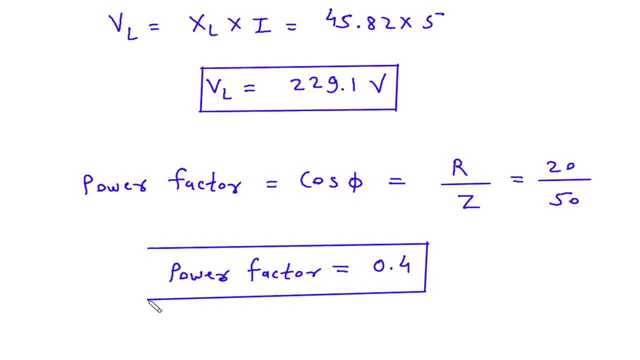 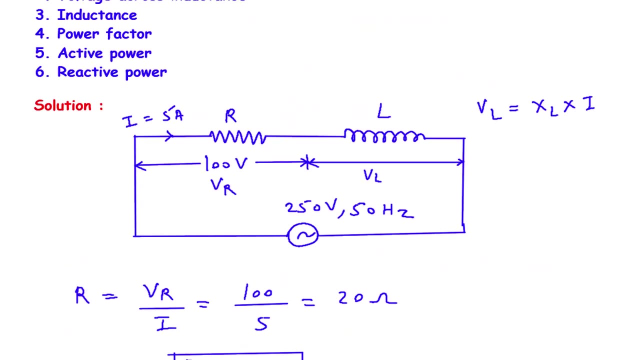 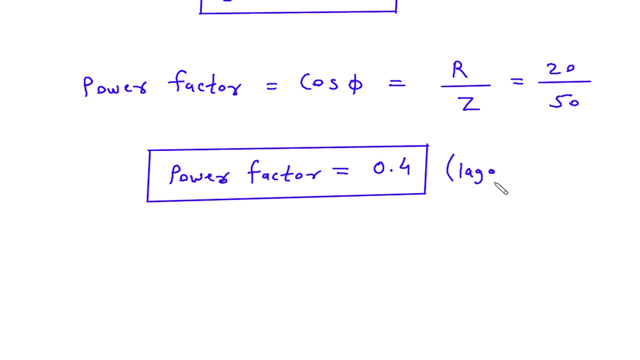 by 50. So this will be 0.4, 0.4, and it is it. have no unit, power factor, have no unit. Then here we can see. it is a combination of resistance and inductance, So the power factor will be lagging. The power factor will be lagging in nature. 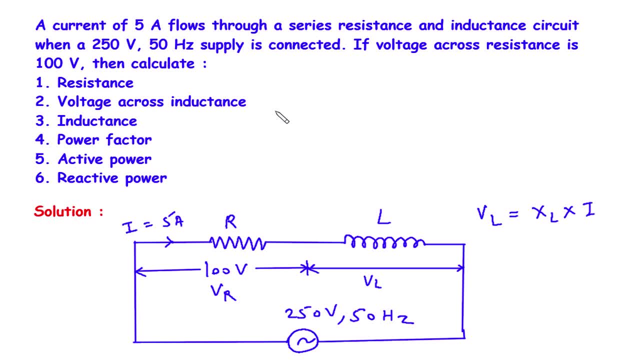 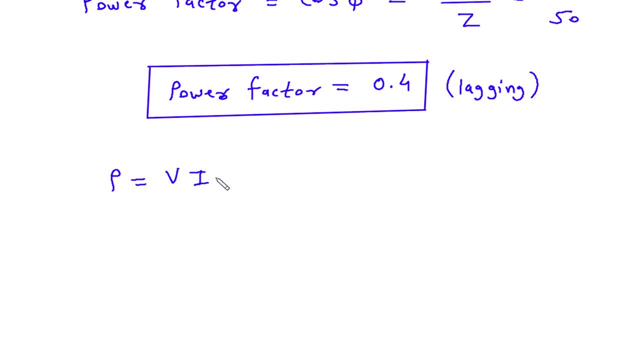 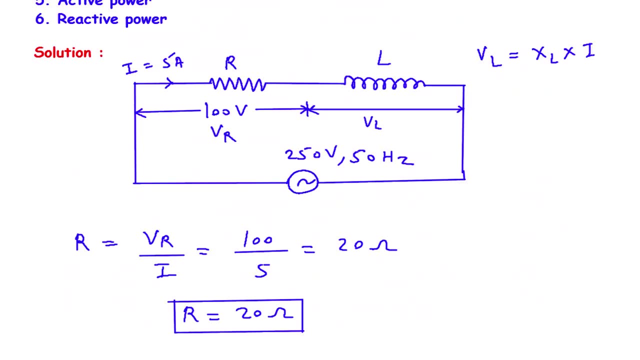 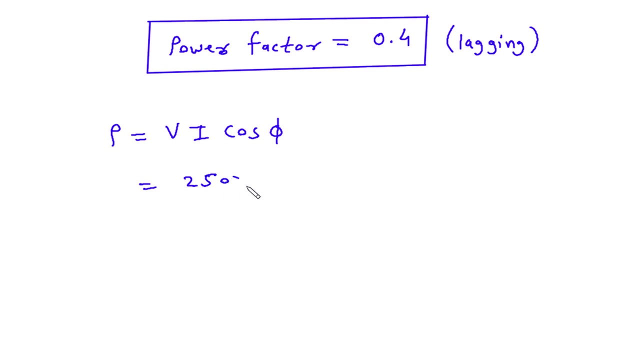 Then next we have to find active power. The formula for active power is: V is equal to V into I, into cos, phi, The value of voltage is given. value of voltage is 250 volt. 250 multiplied by the value of current is. the value of current is 5 ampere. 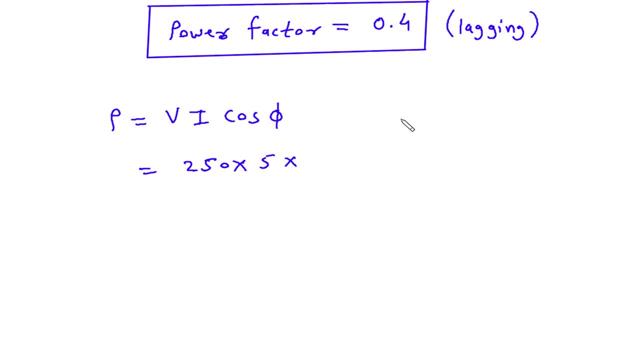 In this case we have to find the value of current. So we have to find the value of current, Then tighten the numeral. This is circuit, when multiplied by cos phi, The value of cost phi, and here we have calculated it as 0.4, 0.4.. 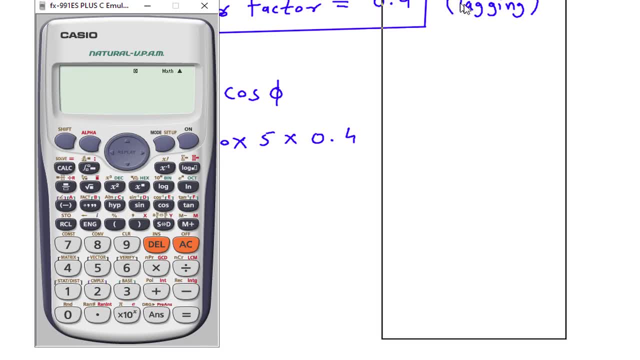 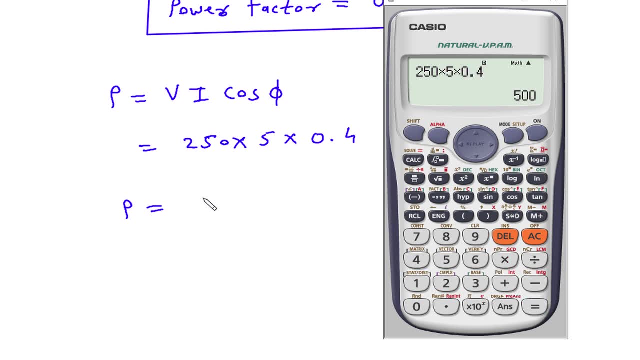 Therefore, power is equal to 250 multiplied by 5. you multiplied by 0.4.. So it is 500.. And its unit will be Vat, because it is power And it is active power. There you keep it for now. OK, Now see, this is 9 electronic circuit. This is V1.relative to security Indicator compositions. it scaled to larger number and it is S time Let us explain this to you. Soetta S might be one all unit matrix, So think of it as simple. here It has shadow as other units. Now we Plus. 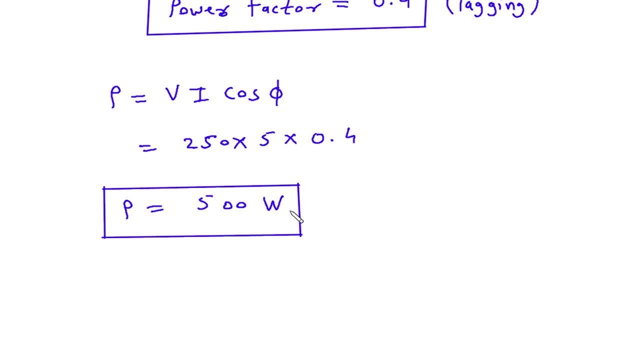 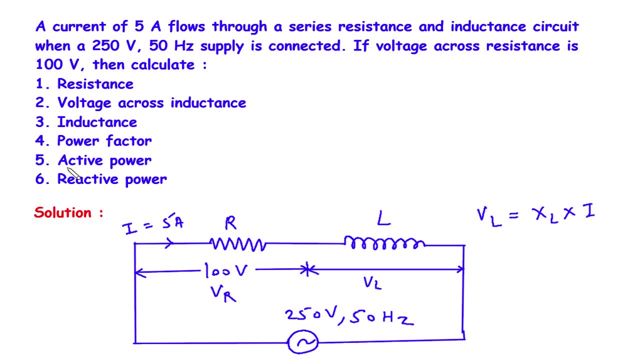 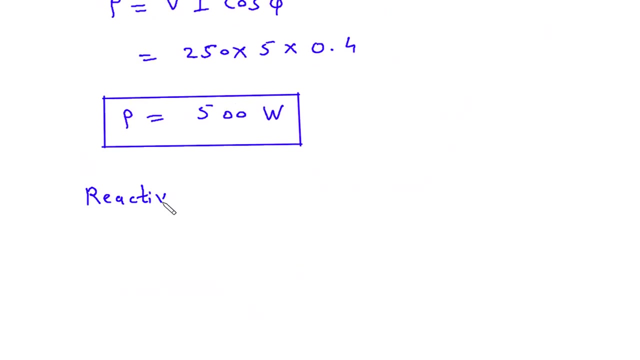 active power, its unit will be wet. Then next we have to find reactive power. Next we have to find reactive power. So reactive power is equal to V into I, into sin phi. Again, the value of voltage is 250 multiplied by value of current, is phi multiplied by. now here this: 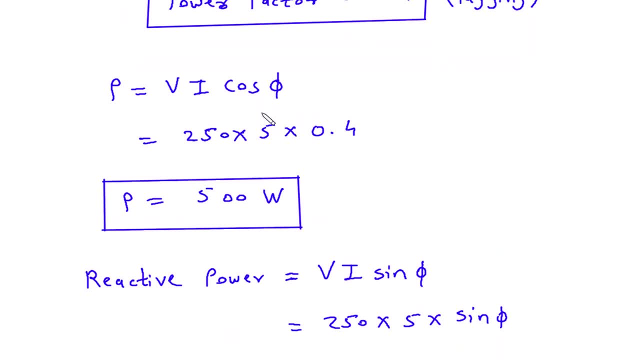 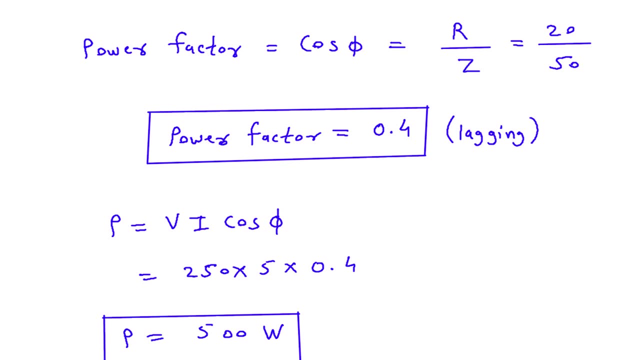 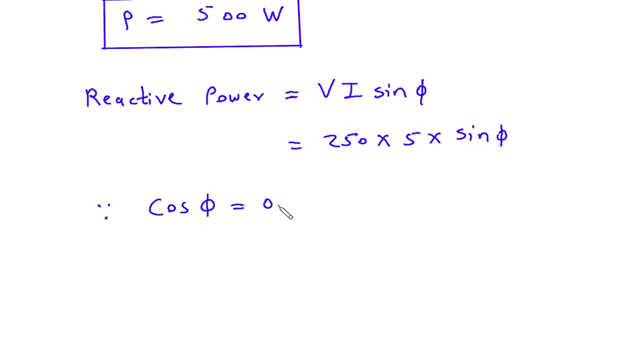 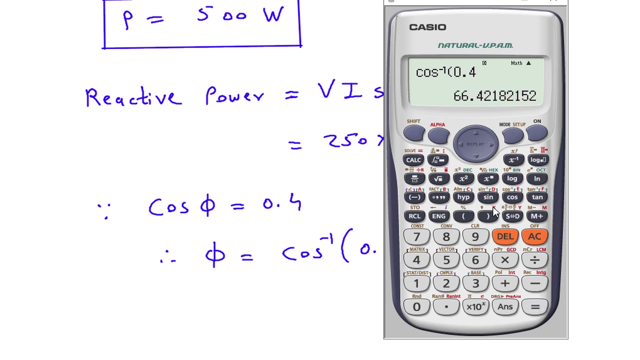 sin phi. Now here we can calculate the value of. from this power factor We can calculate the value of phi. So, first of all, since cos phi is equal to 0.4. So therefore we have: phi is equal to cos inverse of 0.4. So this will be cos inverse of 0.4.. It is 66.42 degree.